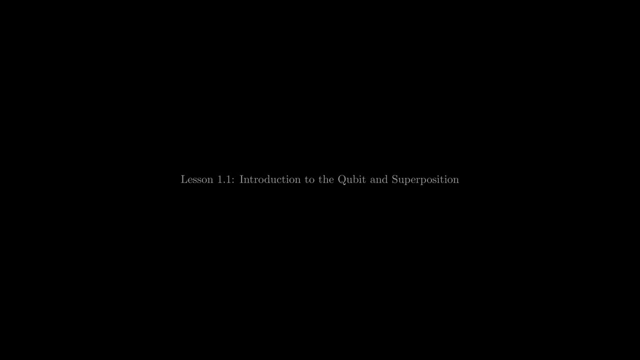 Classical computers use binary 0s and 1s to store and process their data. Quantum computers, on the other hand, use qubits or quantum bits, which can be 0 and 1 at the same time. We have all heard this explanation of quantum computers, but what does that actually mean? 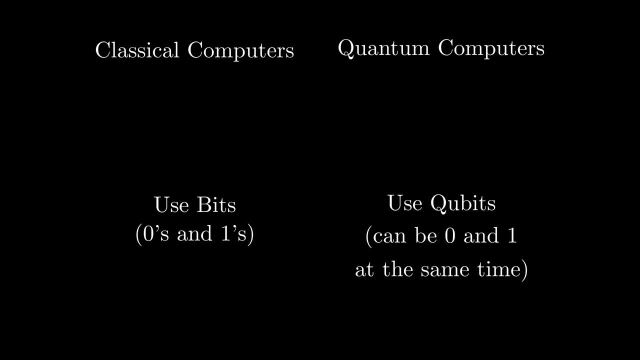 In order to understand what a quantum computer is actually doing, we must look at how we represent them mathematically. Instead of using binary. like classical computers, quantum computers use qubits. Physically, a qubit can be any quantum particle that exists in. 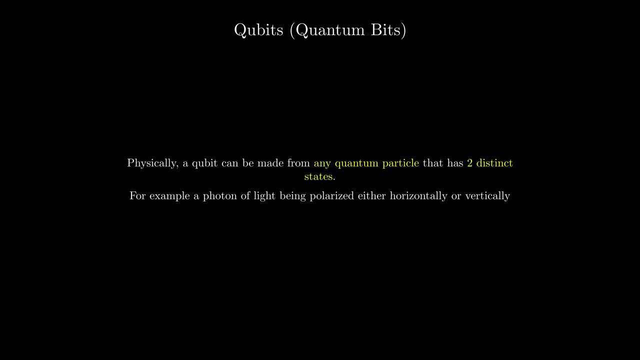 two distinct states, such as a photon of light being polarised either horizontally or vertically. Just like classical computers, we still use 0s and 1s, but in quantum computation we define them instead as the column vectors 1, 0 and 0, 1 respectively. 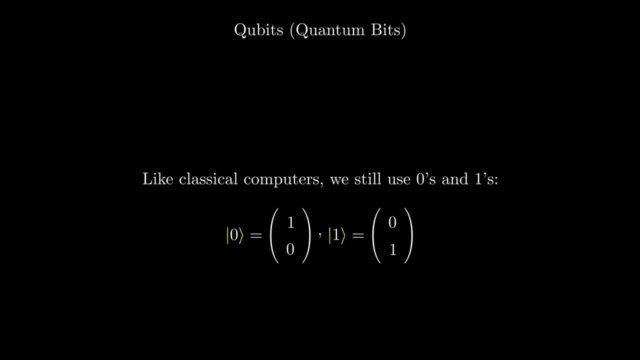 The weird brackets around the 0 and 1 is Dirac notation. We will look more into it later. You may have heard of the term superposition. What it means in quantum mechanics is that a quantum particle is in two states at the same time. So back to our photon polarisation. 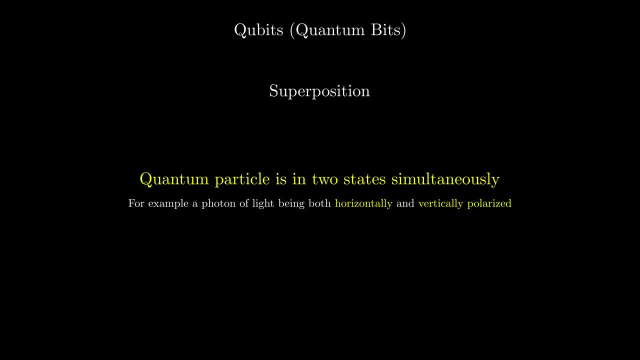 example. this means that the photon is both horizontally and vertically polarised at the same time. In terms of quantum computing, we say a qubit is in superposition if it is both 0 and 1.. Let's look at how we represent qubits mathematically. 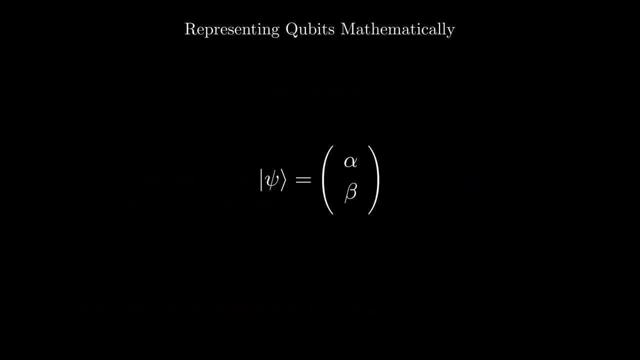 Mathematically we can represent a qubit as a column vector with two elements. The top element indicates how much the qubit is in the 0 state and the bottom element indicates how much the qubit is in the 1 state. The convention for a quantum state is to set it. 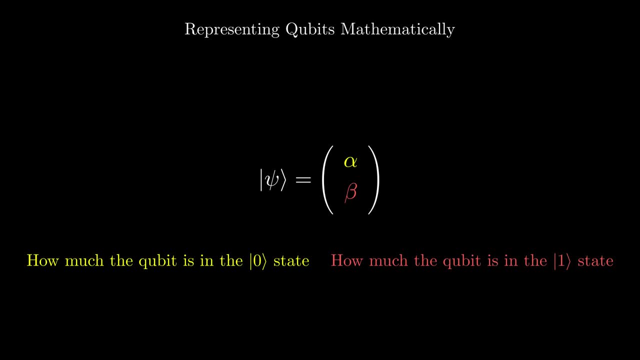 equal to the Greek letter psi. We will talk more about this in the next video. So if we have a qubit in the state 1,, 0,, it now means that it is in the same state as a qubit. It now makes sense why this is 0, since it is all in the 0 state and none in 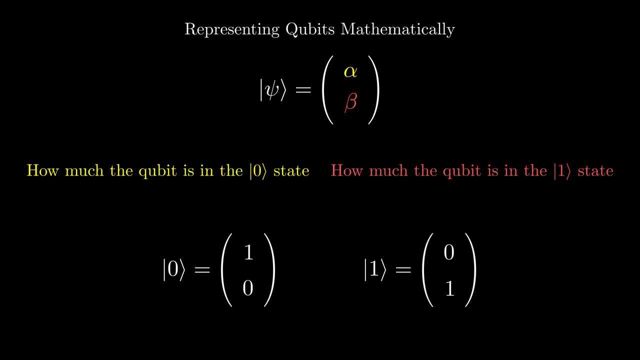 the 1.. We can say the same for a qubit in the state 0,, 1 being 1.. If a qubit is in both the 0 and 1 state, so it has non-zero numbers in the matrix, then we say it is in a superposition. 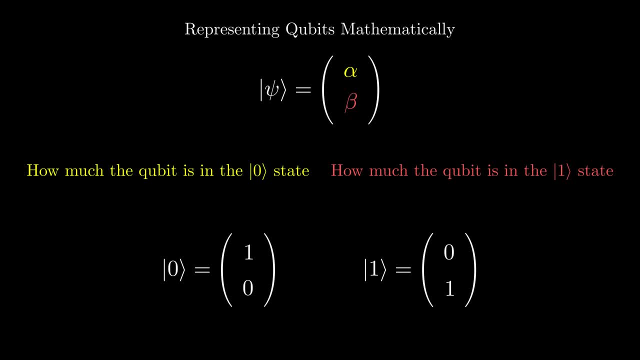 of 0 and 1, since it is both of the states at the same time. So now we know how to represent a qubit mathematically, But how do we measure the qubits? For that we must look at another rule of quantum mechanics. For that we must look at another rule of quantum mechanics. 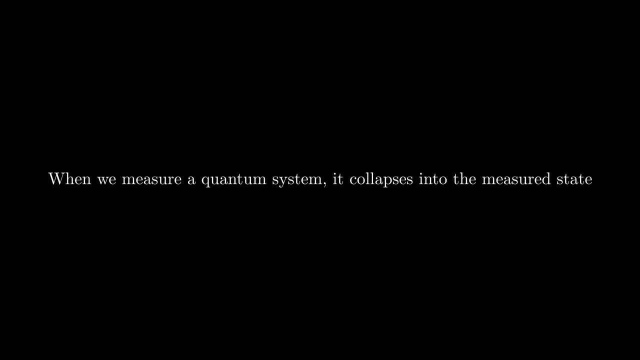 When we measure a quantum system, it changes the state of the system to the measurement. What does that mean? If we go back to our photon polarisation example, if the photon is in a superposition of both horizontally and vertically polarised, then when we measure, 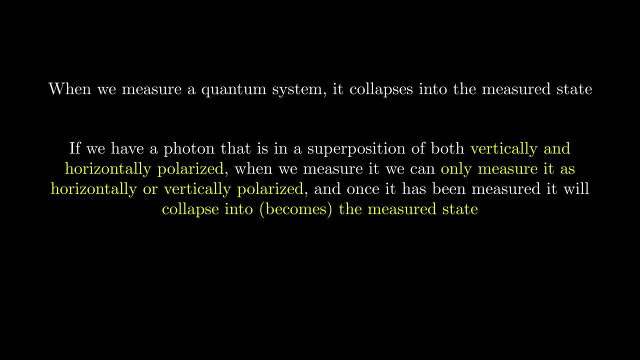 it. we will only measure it as one or the other, but not both, and once it has been measured it collapses into the state we measured. So if it was in a superposition and we measure it to be horizontally polarised, it would. 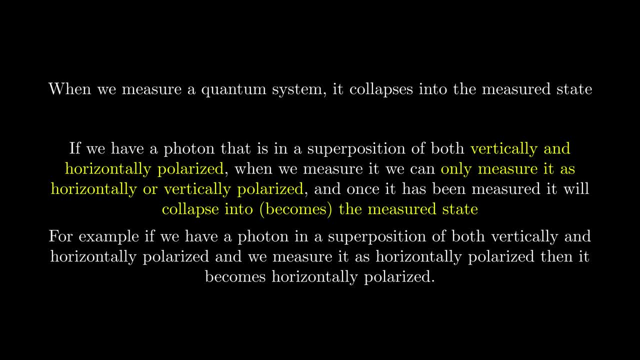 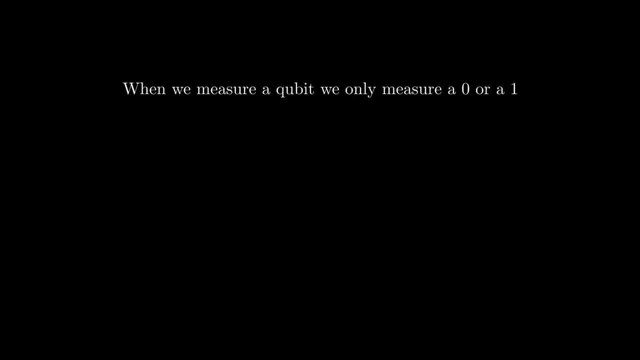 collapse and become horizontally polarised, meaning it is not in a superposition anymore. The same thing happens when we measure qubits. We can only measure a 0 or a 1.. We do not measure how much the qubit is in the 0 state or how much the qubit is in the 1 state. 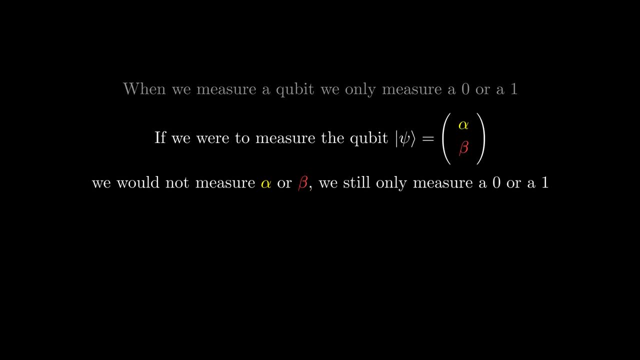 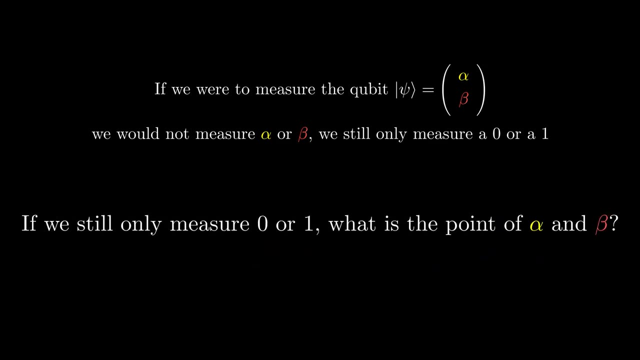 Immediately after measuring a qubit, its state changes to either 0 or 1, depending on the measurement. So what is the point in those numbers telling us how much the qubit is in the 0 state or the 1 state? What those numbers tell us is the probability of measuring. 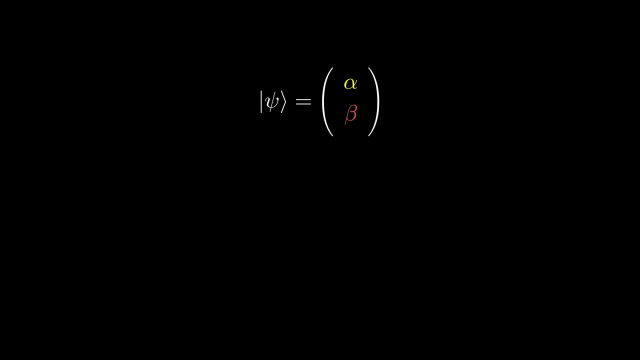 a 0 or a 1.. The probability of measuring 0 is the magnitude squared of the amplitude of the 0 state, and the probability of measuring 1 is the magnitude squared of the amplitude of the 1 state. So for this example, qubit, when we measure it, we have a 75% chance of measuring a 0.. 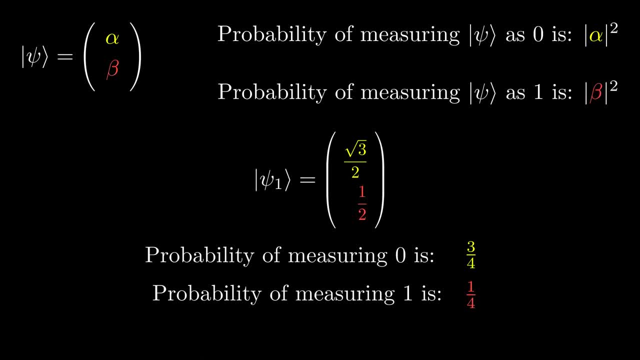 And a 25% chance of measuring a 1.. If we now think about how we defined the 0 and 1 state at the start of the lesson, they should now start to make sense. We stated that 0 was the column vector. 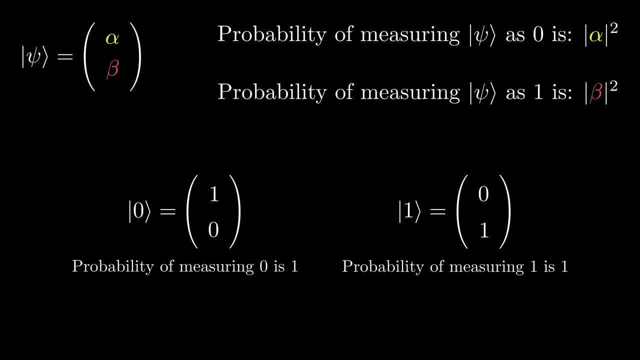 and now we can see why. The probability of measuring 0 is 1,, so it will always be measured as 0. This is the same for the 1 state, Since there are only two possible outcomes when measuring a qubit. the probability of measuring a qubit is 1, and the probability of